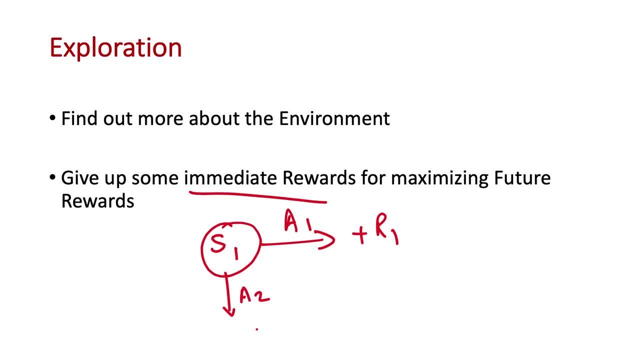 taking some other action A2, it may gain some reward which is equivalent to 2 R1, 2 times R1.. So it has not explored this yet. So this thing is called exploration, and continuing on some known action to get some reward is known as exploitation. 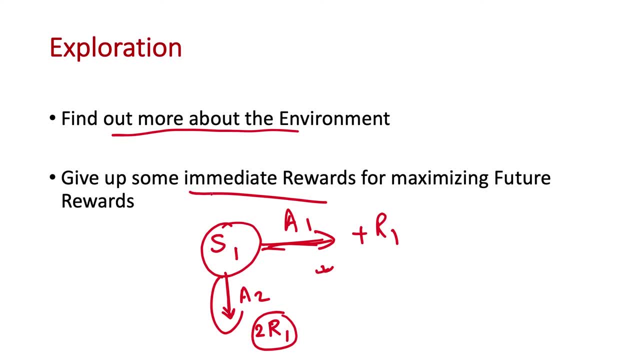 So exploration is finding out more about the environment and it may be possible that this action is not good and it may give some negative reward. So agent has no idea, but it may give some greater reward also. So here it involves giving up some immediate rewards, but if it finds some other action, 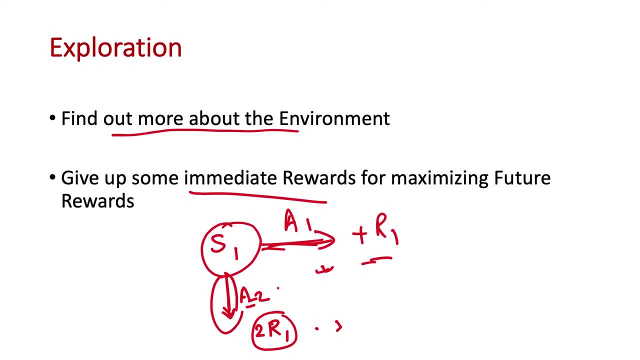 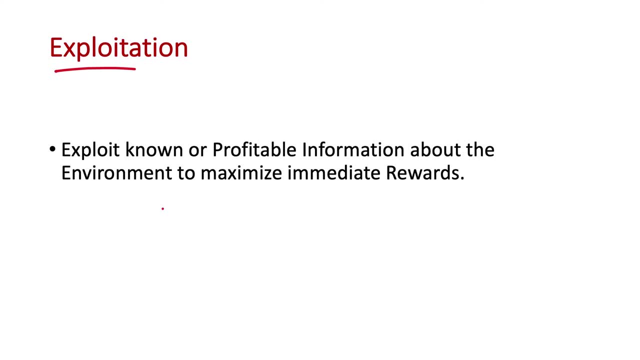 which is more profitable than A1, then in future, in the long term, this will generate more reward. The third concept is exploitation. Exploitation means to use or exploit the known or profitable information about the environment to maximize immediate rewards. So there should be some trade. 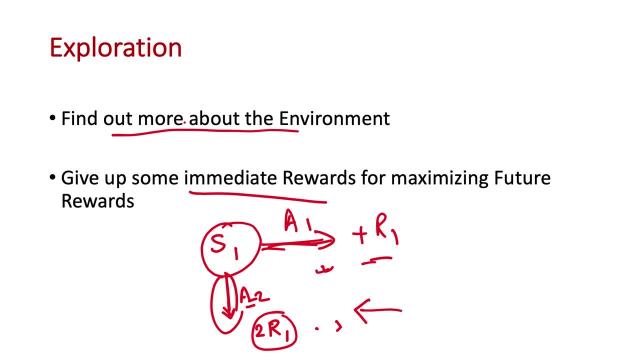 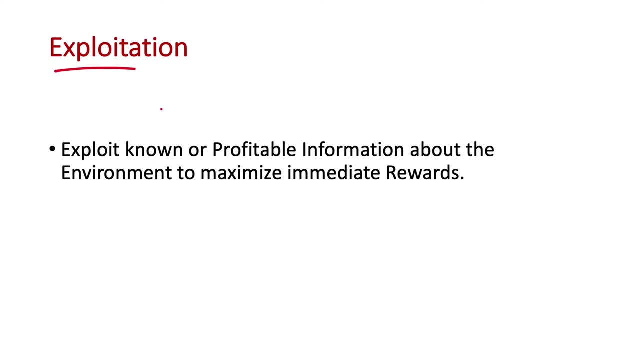 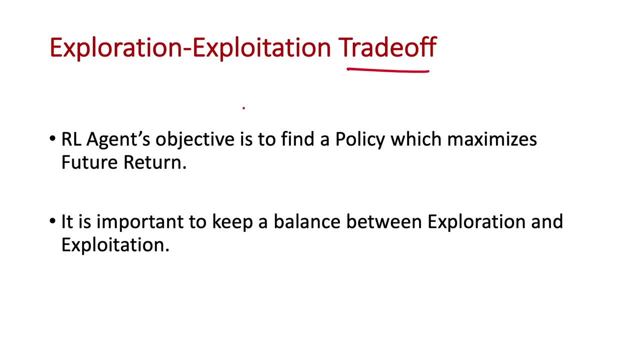 off between these two. One agent should not just go on exploring things and on the other hand, it should also not just keep on taking the same action, because there may be some better action available which will be known only after exploration. So there is a trade-off between exploration and exploitations, and RL agent's objective is to find a policy which will 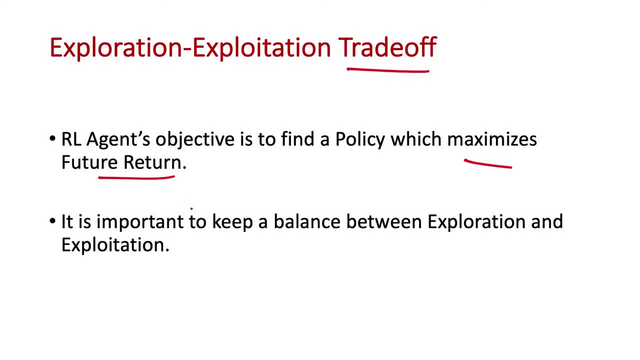 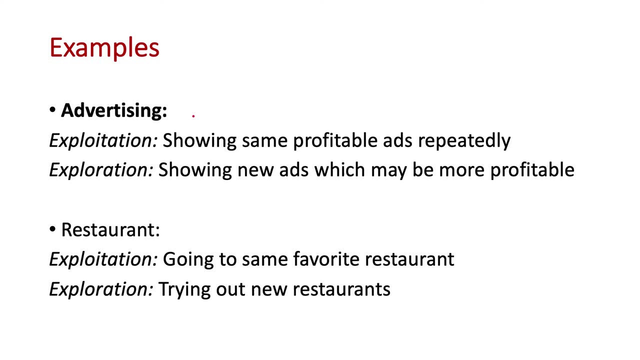 maximize the future return. So it can forfeit some of the immediate rewards, but the future return would be more. So it's important to keep a balance between the exploration and exploitation. Let's see some examples. So if some advertising is popular and some advertisements are, 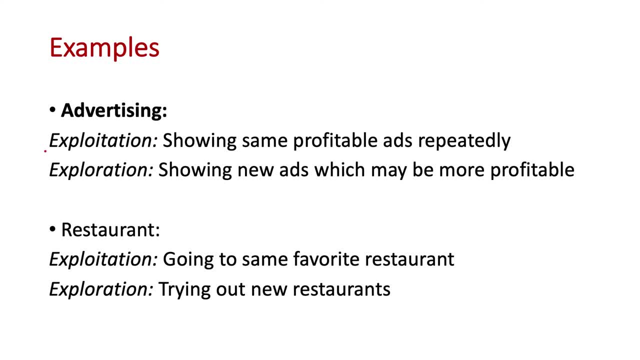 generating good amount of revenue for some company. So exploitation would be showing the same profitable ads repeatedly because it is generating revenue, but exploration would involved showing some new ads which may be more profitable than this earlier ad. So there should be a balance between these two, that how frequently we should show some new ad and try to explore more options.